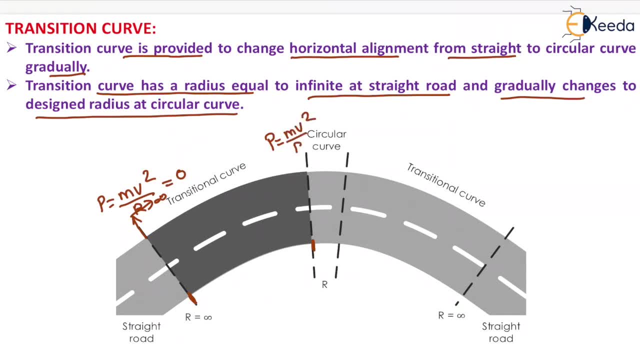 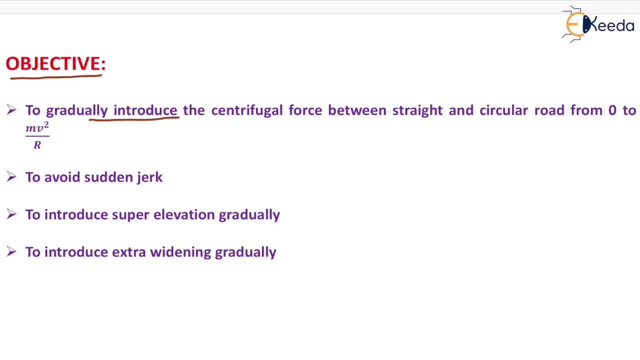 increase from 0 to mv square by r. Now, in this way we had increased the centrifugal force gradually. Now the objective of providing the transition curve to gradually introduce the centrifugal force between straight and circular road from 0 to mv square by r, which 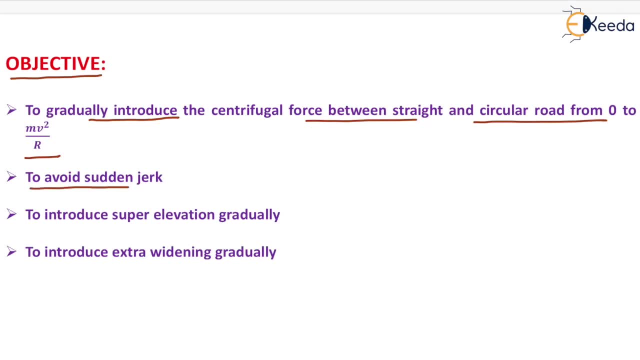 we had seen already. second one is to avoid sudden jerk. the next one is to introduce super elevation gradually and the last one is to introduce extra widening gradually. now, if we provide a transition curve at the junction of straight alignment and circular curve, then we will avoid sudden jerk. 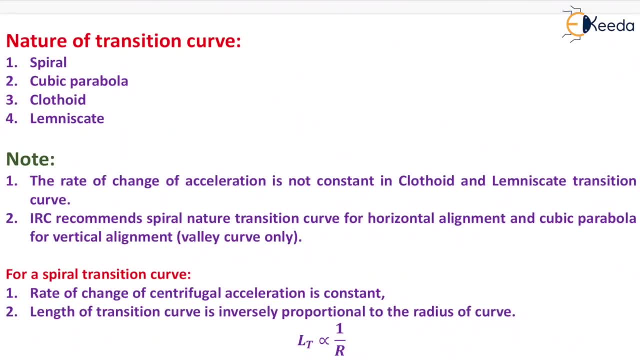 condition. now, nature of transition curve is generally spiral, cubic, parabola, clothoid and lemniscate curve. now note is written here that the rate of change of acceleration is not constant in clothoid and lemniscate transition curve. that's why they are not used as a transition curve. 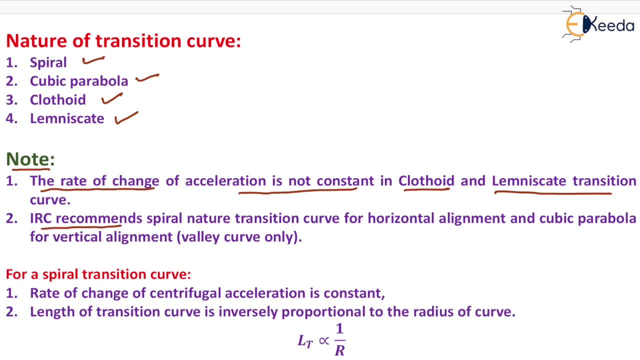 the second one is: irc recommends spiral nature transition curve for horizontal alignment and cubic parabola for vertical alignment. now, this is very important from the gate point of view as well as from the other exams point of view, that the spiral nature transition curve is generally provided for horizontal alignment and cubic parabola is. 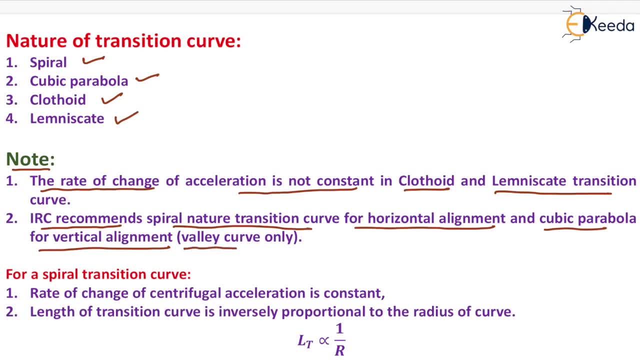 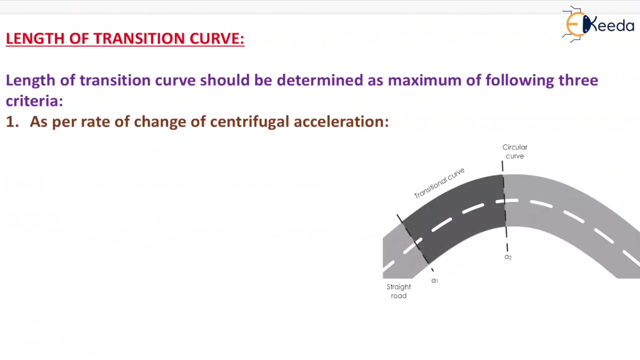 generally provided for vertical alignment, that is, valley curve only. for a transition curve, the rate of change of centrifugal acceleration is constant, as well as the length of transition curve is inversely proportional to the radius of the curve which is shown here. that is, lt is inversely proportional to radius of the curve. now we have to find the. 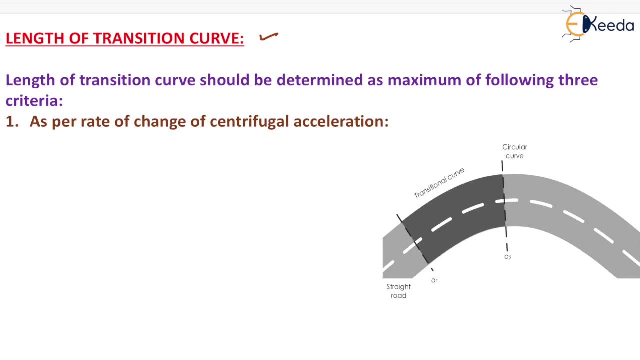 length of transition curve. now it will be generally determined from the three criterias. the first one is as per the rate of change of centrifugal acceleration. now, as per the first criteria, here straight road is shown and here a circular curve is shown. now, in between the straight road and circular curve there will be a transition curve, which is provided. 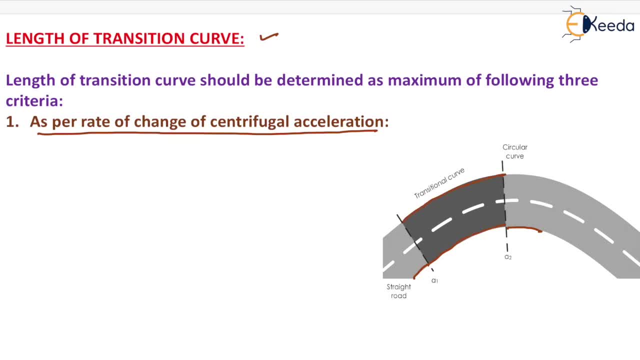 here like this now: here the acceleration is a1 and here the acceleration is a2. now we will find the value of length of transition curve. the rate of change of centrifugal acceleration will be equals to a2 minus a1 upon time. now we all know that P equals to ma, that is mass. 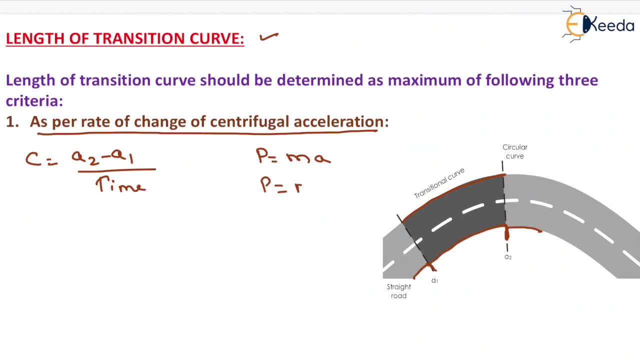 into acceleration as well. as p is equals to MV square by r. that will be the centrifugal force. on equating these two, we will get A is equals to V square by r. now we will put the value here. that will be the present Esta La shocked me. I actually not. I am in the center. when the velocity will be filling up. then I will calculate it in representation value. A carbine mass will be equal to ma divided by E, for coefficient will be Equal to P against mv square by r. that will be the centrifugal force. on equating these two will will get Midwest behandlable. 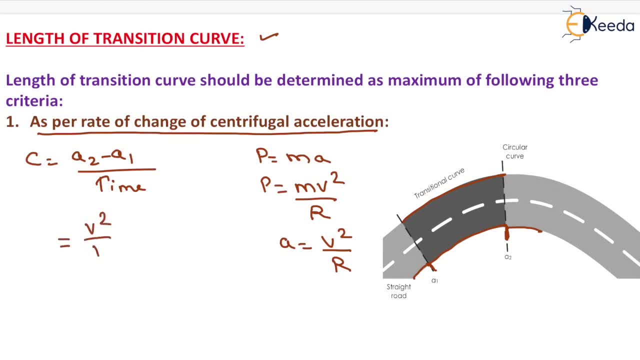 of electronic and electronic. please watch this video. spoken name is V square by R minus 0, because at this point the radius is infinite. and if radius is infinite, then we will put this value as infinite. that is this value, so acceleration will be equals to 0, and if we put the value of R equals to R, that 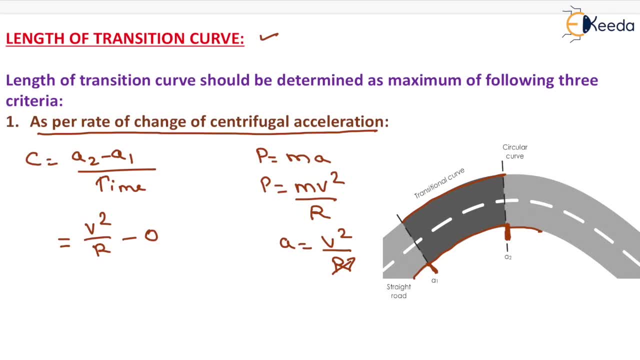 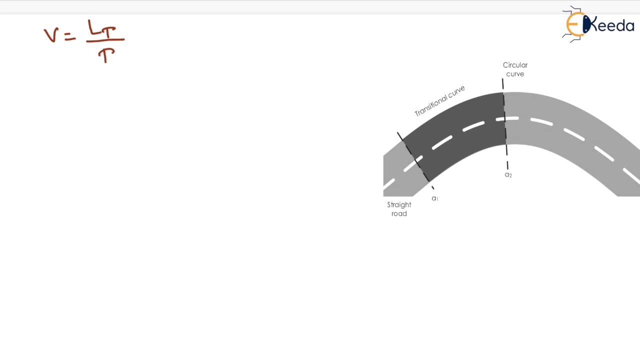 is for this point, then acceleration will be equals to V square by R, that is the value of A2, and we will divide this value by time, that is capital T. so it will be the value of centrifugal acceleration. now it will be equals to V square upon RT. speed will be equals to distance upon time, so it will be equals. 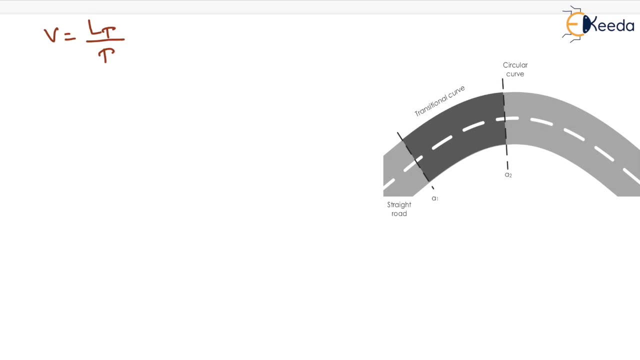 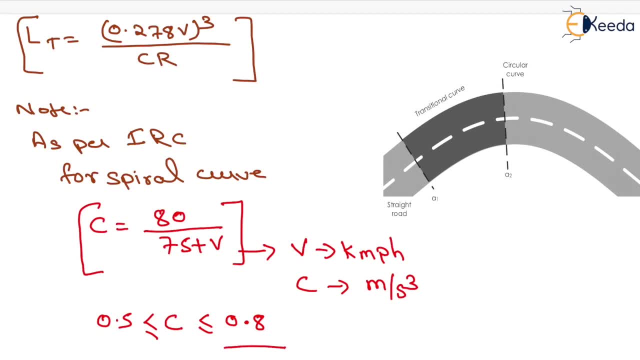 in the equation that is C equals T, and we will put this value in the equation that is C equals T, and we will put this value in the equation that is C equals T, and we will put this value. Now, this is the length of transition curve as per the first criteria.